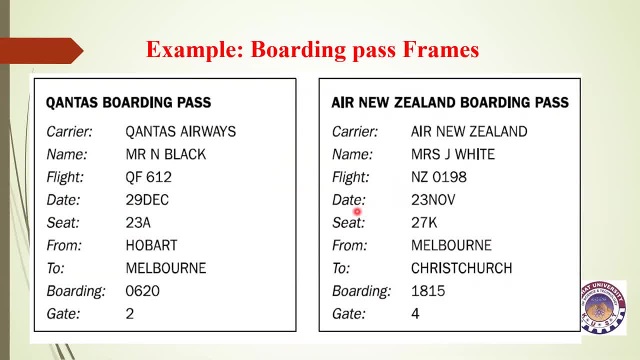 frames with knowledge about airline passengers. Both frames have the same structure. Qantas Airways Limited is the flag carrier of Australia and is the largest airline by fleet size. This figure shows a boarding pass of the Qantas Airways. Here the frame name is Qantas Boarding Pass. 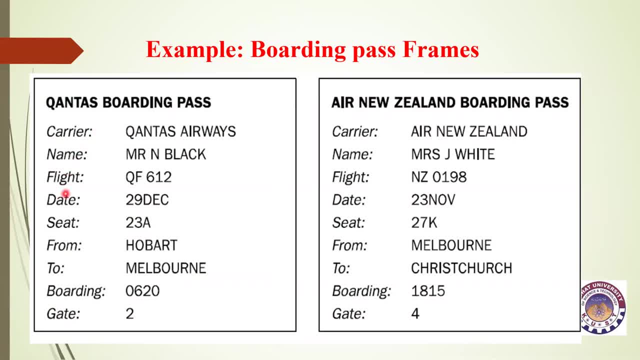 Carrier name, flight date, seat, and all these are the slots of the frame. A slot carrier, for example, has value- Qantas Airways- and a slot gate has value too In some cases. instead of Qantas Airways, a slot may have a procedure that determines the value. 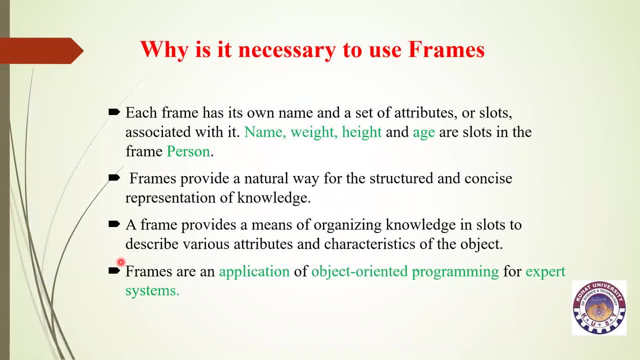 A frame is a record-like structure which consists of a collection of attributes and its values that describe information about an entity in the world Means. each frame has its own name and a set of attributes are slots associated with it. Name, weight, height and age are slots in a frame of person. 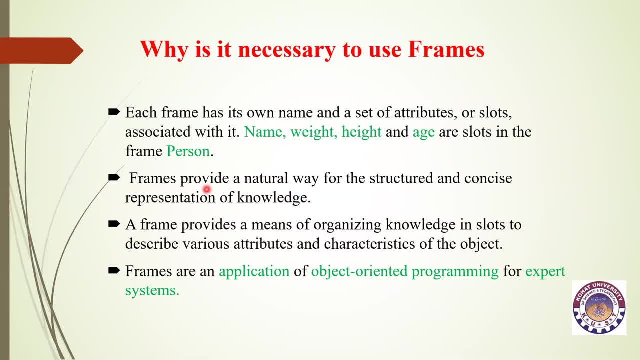 Frames provide a natural way for the structured and concise representation of knowledge In a single entity. a frame combines all necessary knowledge about a particular object or concept. A frame provides a means of organizing knowledge in slots to describe various attributes and characteristics of the object. 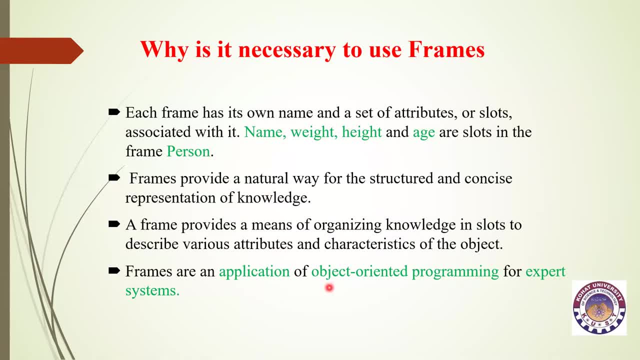 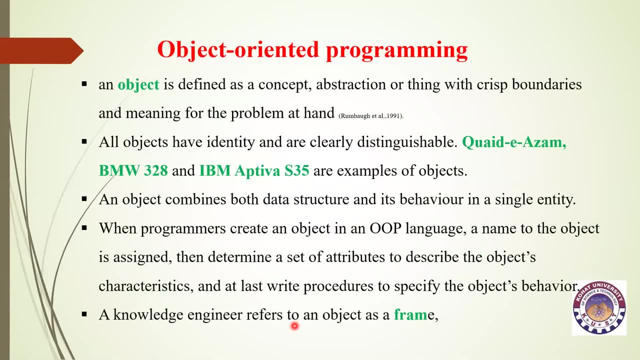 Basically, frames are an application of object-oriented programming for expert system. So what is object-oriented programming? Object-oriented programming can be defined as a programming method that uses objects as a basis for analysis, design and implementation. In object-oriented programming, an object is defined as a concept. 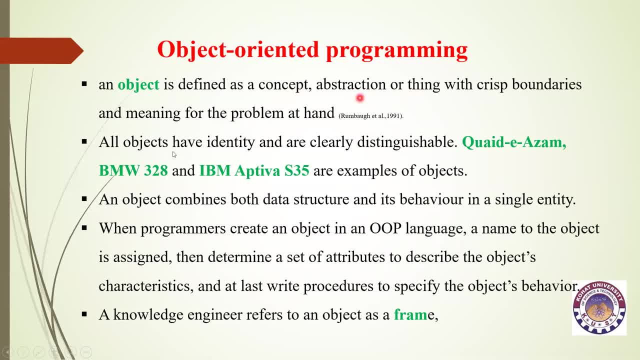 Abstraction are things with crisp boundaries and meaning for the problem at hand. All objects have identity and are clearly distinguishable. Kaidyasam BMW 328 and IBM Aptiva S35 are examples of objects. Objects can be anything, or any entity or any concept present in the world. 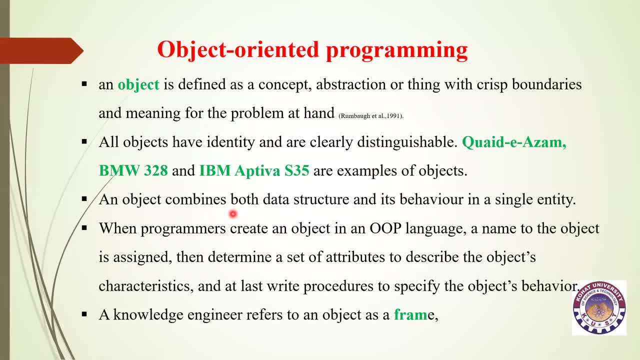 An object combines both data structure and its behavior in a single entity. Object-oriented programming offers a natural way of representing the real world in a computer. When programmers create an object in an object-oriented language, they first assign a name to the object, then determine a set of attributes to describe the object's characteristics. 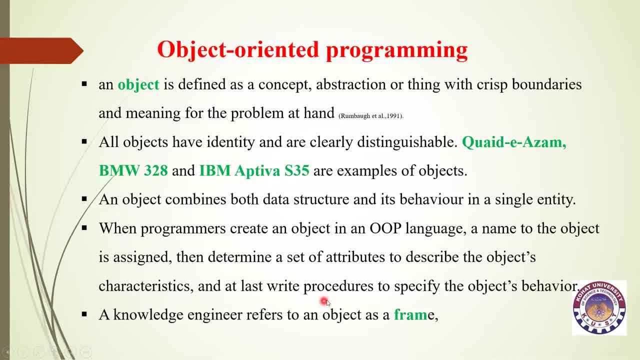 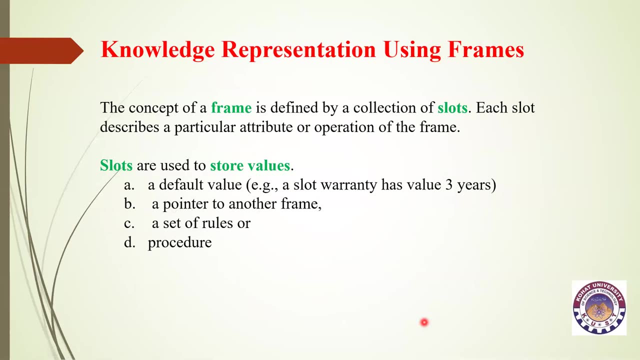 and at last write procedures to specify the object's behavior. A knowledge engineer refers to an object as a frame. The concept of a frame is defined by a collection of slots. Each slot describes a particular attribute or operation of the frame. Slots are used to store values. 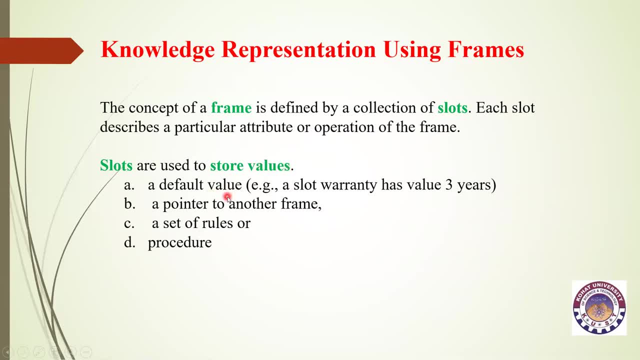 A slot may contain a default value. Example of default value is warranty of a laptop, which is usually 3 years, So this shows the default value. A slot may contain a pointer to another frame. A slot may be a set of rules or procedures. 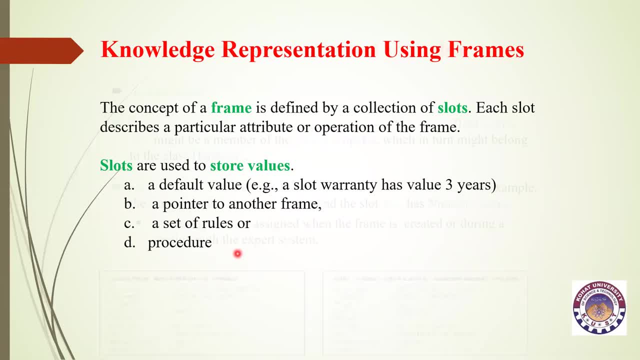 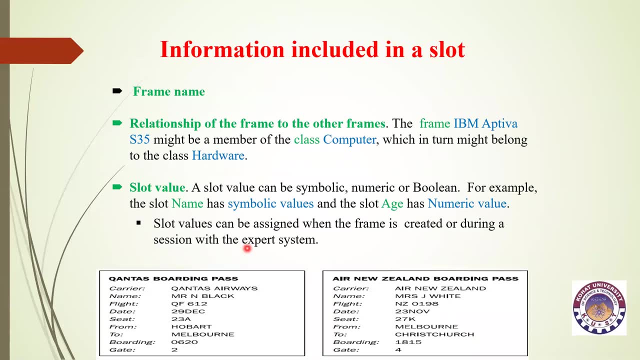 by which the slot value is obtained. In general, slots may include such information as frame name, which is actually the entity, concept or an object present in the world. the relationship of the frame to other frames. the frame IBM Aptiva S35 might be a member of the class computer. 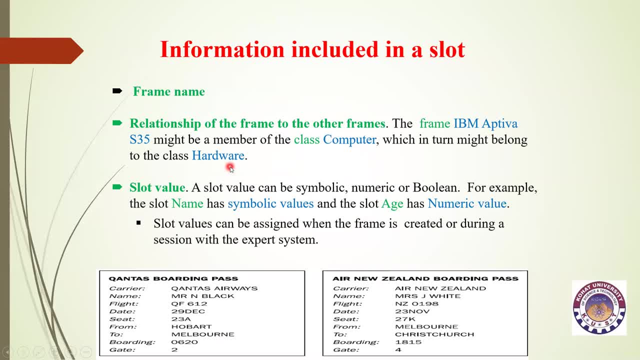 which in turn might belong to the class hardware. So this represents the relationship of one frame to the other frame, a slot, have a slot value. a slot value can be symbolic, numeric or boolean. for example, the slot name has symbolic value and the slot age has numeric value. 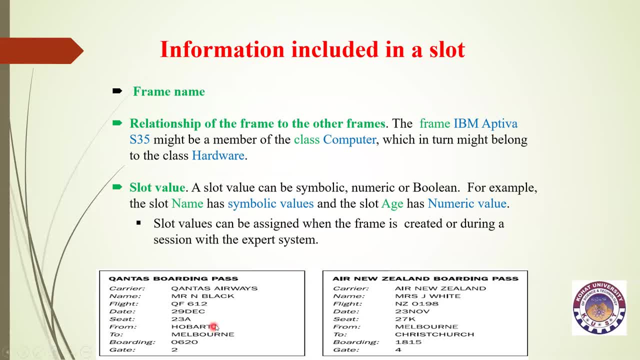 consider the frame in this figure. the slot name has symbolic values and the slot gate has numeric values. slot values can be assigned when the frame is created or during a session with the expert. system means the experts. the expert will suggest the names, the names to the to the engineers project. to the project engineers. 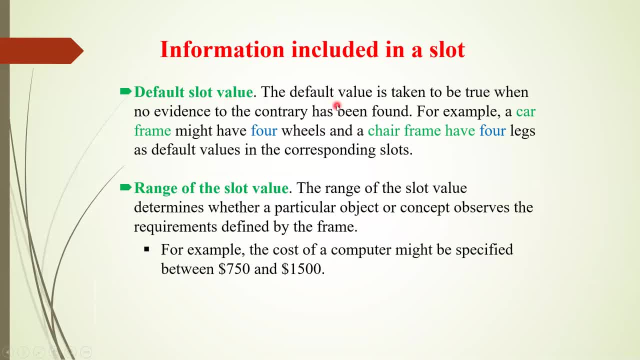 default slot value. the default value is taken to be true when no evidence to the contrary has been found. for example, a card frame might have four wings and a chair frame have four legs, so these are default values. interest in the corresponding slots: a car must have four wheels and a chair must have three- four legs, so this is default value. 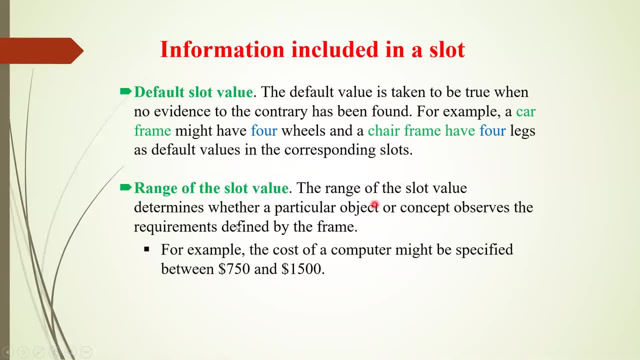 range of the slot value. the range of the slot value determines whether a particular object, our concept, observes the requirements defined by the frame and, for example, the cost of a computer might be specified between some range. for, for example, the range may be 750 and the range may be in between 750 and 1,500. 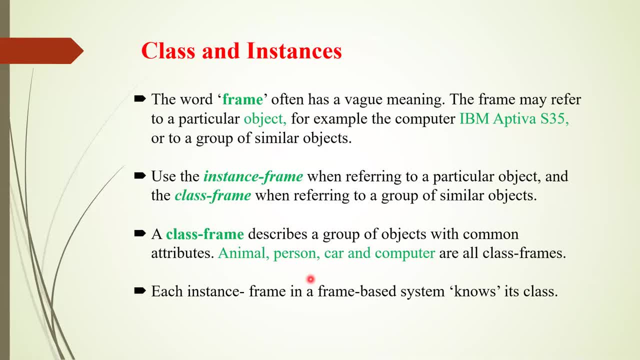 dollars. so what are the class and instances? the word frame is called the Metroid гр wards on the world frame you can see the librarian runs it and Hidden. I am ensuring that my interface, or the git, because our functions are needed- is driven 저는. 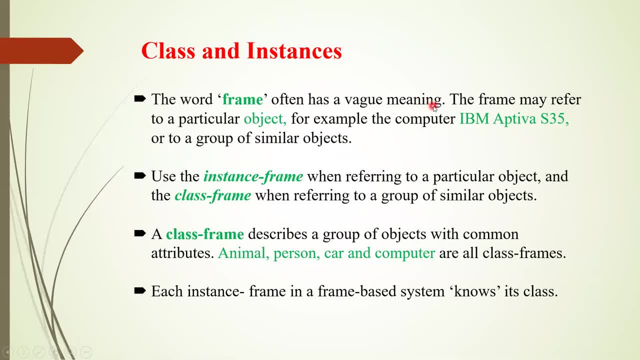 information flow is a provision to the user. input is also a requirement to heartfelt 25mm at the analysis, as well as можно snacking, if you like. it is a reference to our has a vague meaning. the frame may refer to a particular object, for example the. 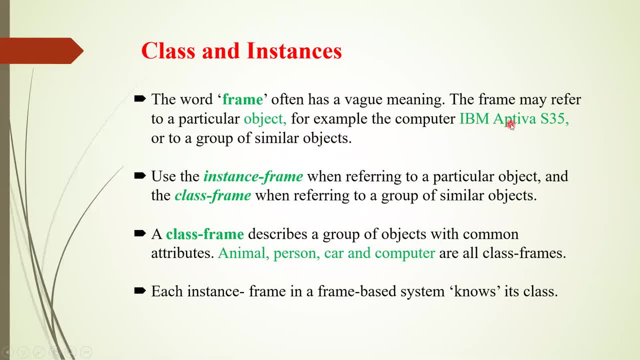 computer IBM Activa S35 are to a group of similar objects. to be more precise, use the instance frame when referring to a particular object and the class frame when referring to a group of similar objects. a class frame describes a group of objects with common attributes, for example, animal person, car and. 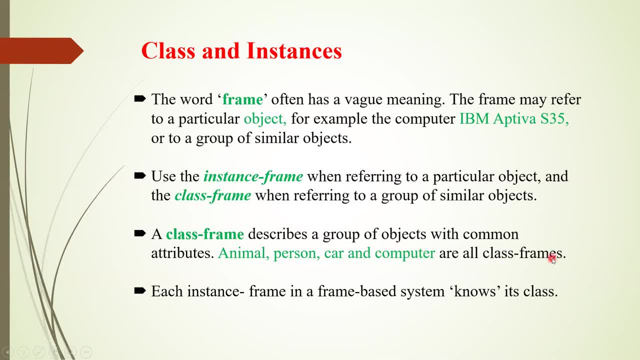 computer are all class frames. each frame in a frame based system knows its class. in other words, the frames class is known is the known property of the frame: animal, person. these are class frames and a particular person named Ahmed, for example, is an instance of frame. so person is a class and a mother is the instance of that. this class for 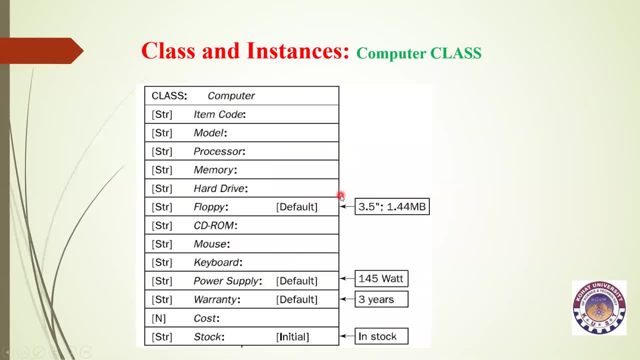 some class person. this figure is illustrates frames describing a class computer. so the class is computer and these are the slots are. you can see these are the attributes are characteristics of a computer. item code model: memory: hard drive, floppy. floppy has a default value. you of this CD-ROM. mouse, keyboard. power supply has a default value of 145 watts. 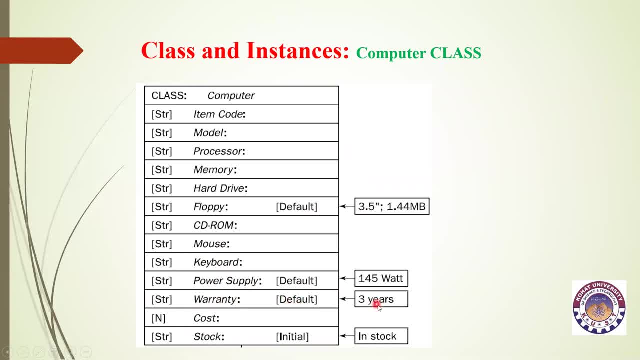 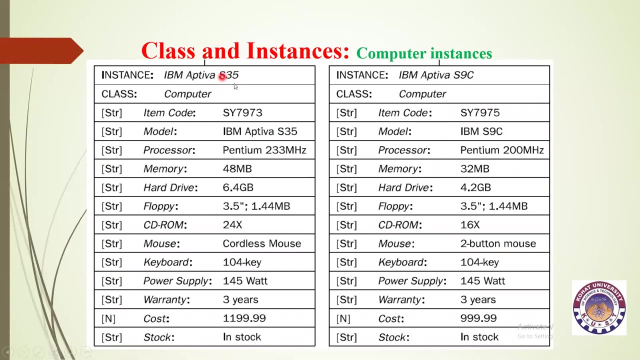 warranty is a default, has a default value of three years cost stock. so this is a class computer. in class computer we have only slots, whereas an instance like IBM Activa S35 is an instance of class computer. so it has the same attributes of the class computer but has different and has associated values. similarly IBM. 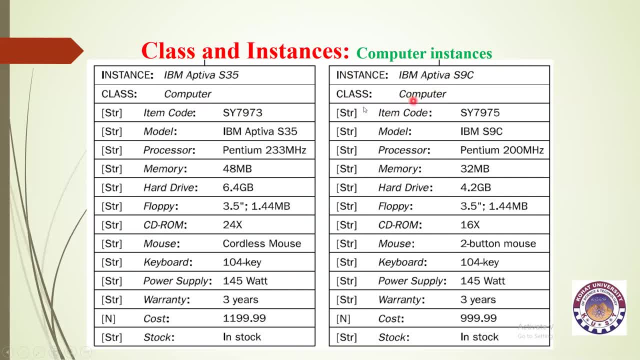 Activa S9C is another instance of a class computer, and it also has the same characteristics, but the associated values are different from this instance to this. so here we can say that two types of attributes are here are used here: string for symbolic information and numeric for domain data. 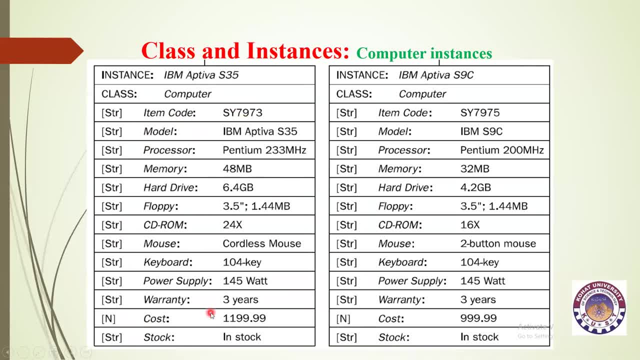 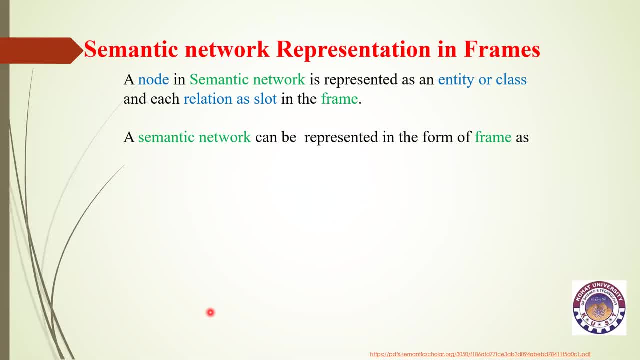 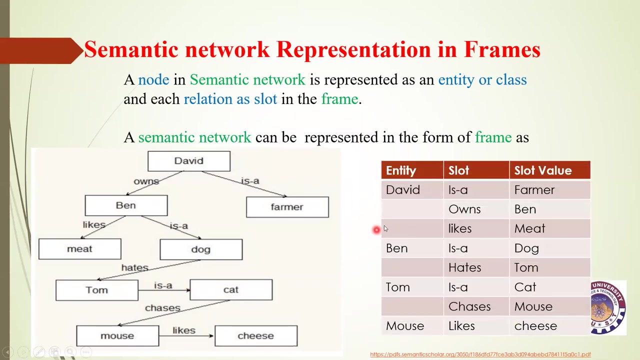 you. this slide shows the semantic network representation in frame. a node in semantic network is represented as an entity or class and each relation as slot in the frame, as a. a semantic network can be represented in the form of frame, as this is a semantic network and this is the frame of this semantic networks. so 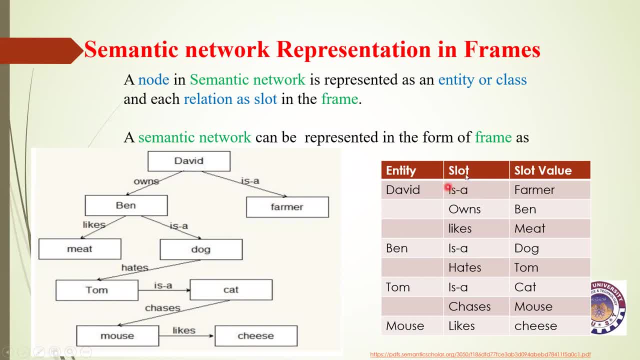 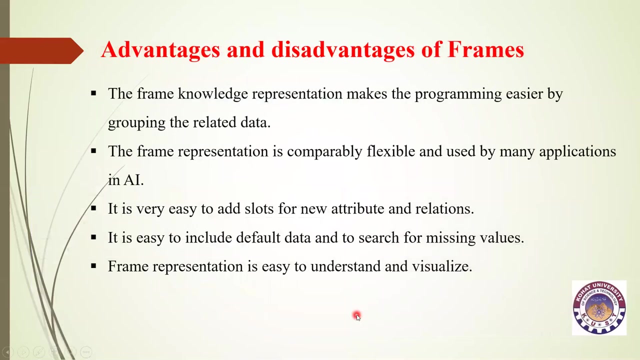 david is a farmer, is a is a slot, our attribute, or shows a relation, and farmer is the slot value david owns. when again own shows a relation which david has with ben tom is a cat, tom chases mouse, and so on. some of the advantages and disadvantages of a frame based knowledge representation method. 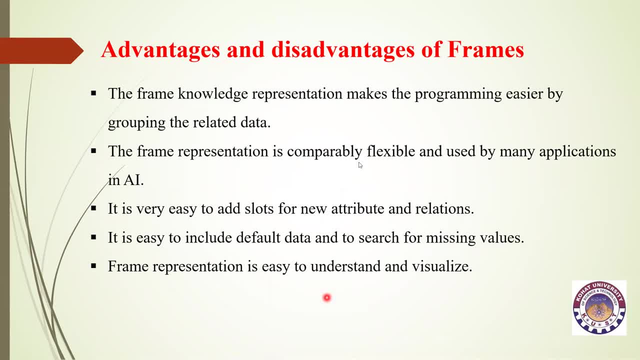 are given in this slide. the frame knowledge representation makes the programming simpler by grouping related data and is therefore used by many applications in in the artificial intelligence. it is very easy to add slots for new attributes and relations. it is easy to include default data and to discover the